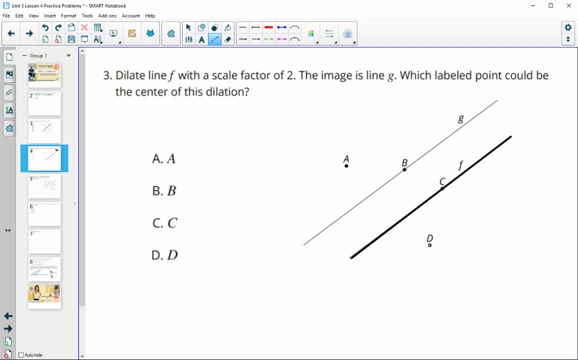 position? Okay, it's one. So what's giving dilated point? So really the only option here would be point D, And if we did just kind of draw, looking at this, we could see that this distance here and then this distance here from D to G, so like this whole thing, versus from D to F, appears to be two times bigger. So 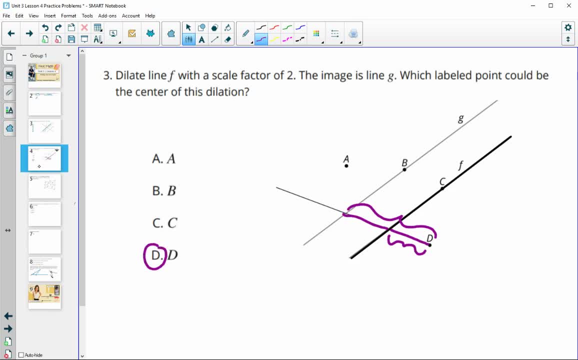 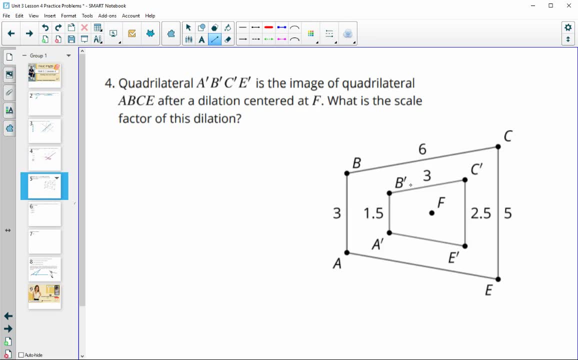 D is the only option there for a center of dilation. Number four: quadrilateral A prime B prime C prime E. prime is the image. So this inner part is the image of the outer part after a dilation around F. So what is the scale factor of this? 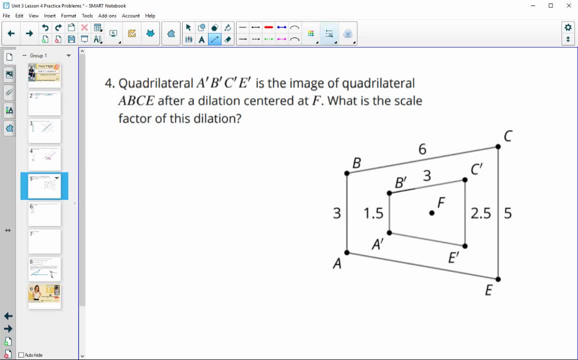 dilation. So, remember, we want to take the new measurement. So if we were to take the new measurement, we would want to take the new measurement of the measurement from the new shape and divide it by a measurement from the original. And we want to 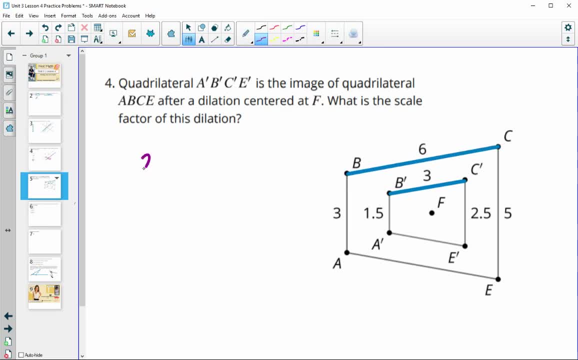 make sure that we're doing corresponding parts. So we're going to take B prime, C prime and divide that by B C and that's going to get us a scale factor of one half. And you could certainly have done other sides. So you could have compared A prime, B prime to AB and done 1.5 divided by 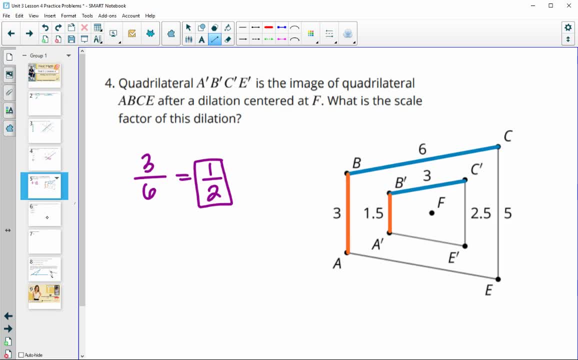 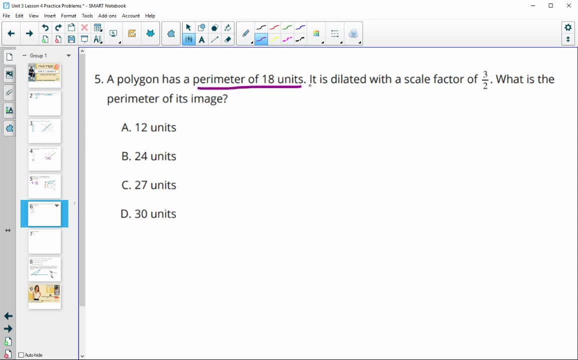 3 or 2.5 divided by 5 would have gotten you the same scale factor, Number five. a polygon has a perimeter of 18 units and it's dilated with a scale factor of three, half, What is the perimeter of the image? So remember perimeter. 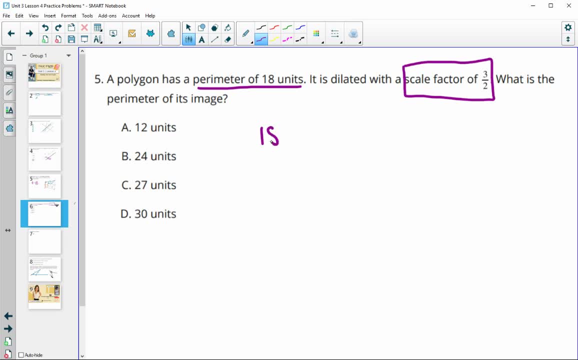 dilates at the same scale factor as the sides. So if the original perimeter is 18, we can multiply that by the scale factor and get our new perimeter. So 18 times 18 is 18.. So if the original perimeter is 18, we can multiply that by the scale factor and get our new perimeter. So 18 times 18 is 18.. 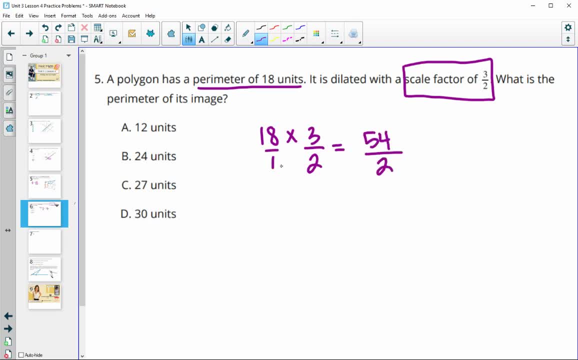 15 times 3 is 54, and then we have divided by 2.. And 54 divided by 2 is 27 units. Number six asks us to solve the equation, So we will just do some cross multiplication here. So x times 4 is 4x, and then 7 times 10 is 70. So we know that the cross products equal each other. 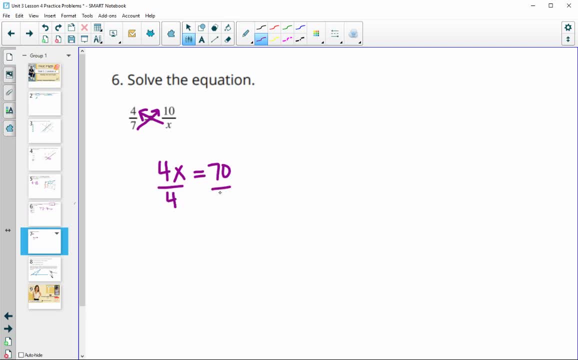 So 4x equals 70. Then we'll just divide by 4, and we get x equals 70 divided by 4, which we could divide both by 2 and simplify to 35 halves, or, if you want a decimal form, that would be 17.5.. 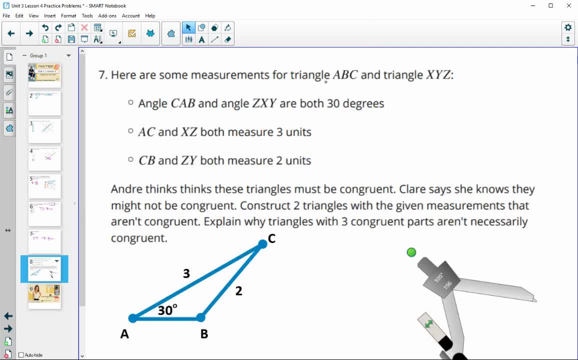 All right. so in number 7, they give us some measurements for triangle ABC and XYZ, and so I've drawn those measurements here into triangle ABC so we can see them. And it says that Andre thinks that the two triangles will be congruent to each other. 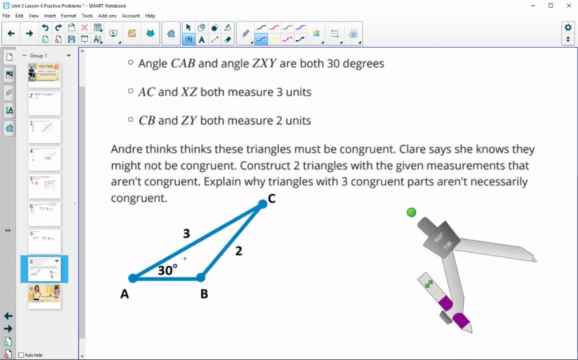 with these measurements, and so I've only drawn one triangle so far. but we can see that the two sides that are given to us do not contain the angle, so the angle is not between those two sides. So, if you remember, that is not going to guarantee that the two triangles are congruent, okay. 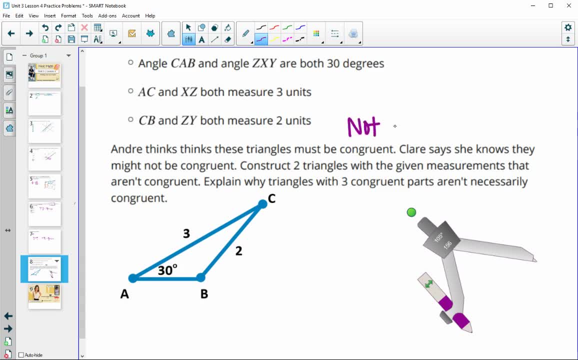 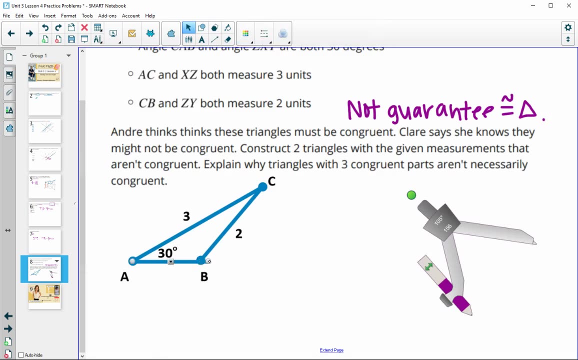 So this is definitely not going to guarantee So the two sides are going to be congruent triangles, and so let's look at why. So this is, why is this not going to work? So we know that this angle needed to stay the same, so they gave us a 30-degree angle. 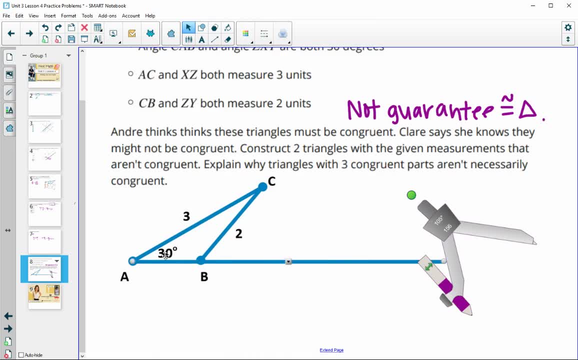 Well, I'm just going to extend this line because that's still a 30-degree angle there. so I haven't changed that measure and I'm going to leave this 3 the same. but what I'm going to look at here? 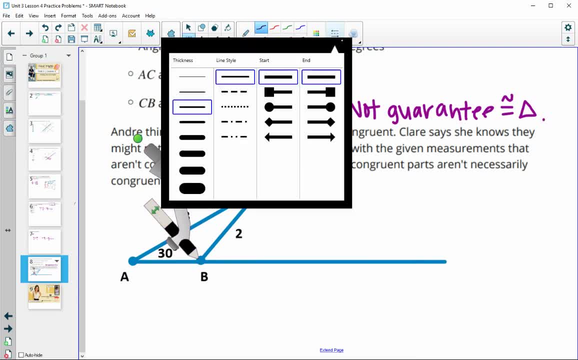 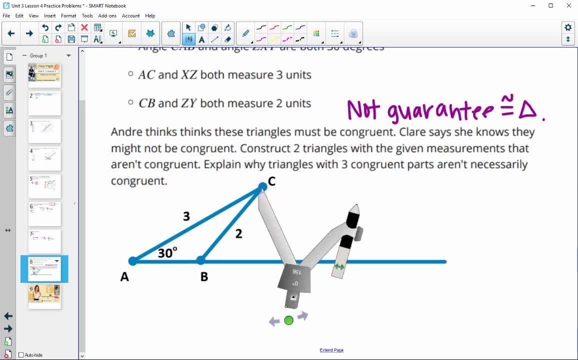 What I've done already is I'm going to use my compass so that I can look at, like, all of the lengths that are 2.. So this would be all of the side lengths that are 2.. So I'm just going to kind of rotate this here and see where it crosses on this other line. 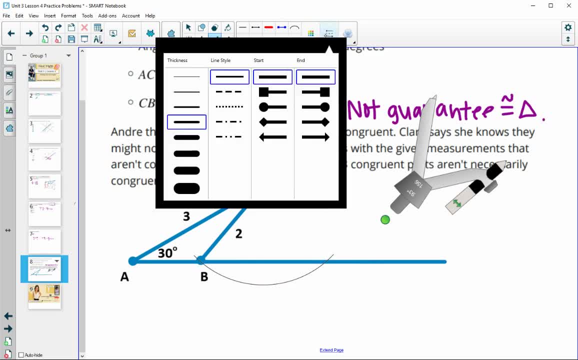 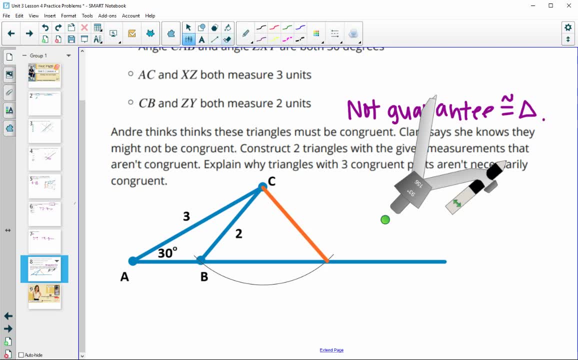 and when I go to draw this segment in here, then we know that this segment is going to look the same. We know that this segment is going to look the same. We know that this segment is going to look the same segment will be equal to this one, since it was created by a circle, So I know that this length-